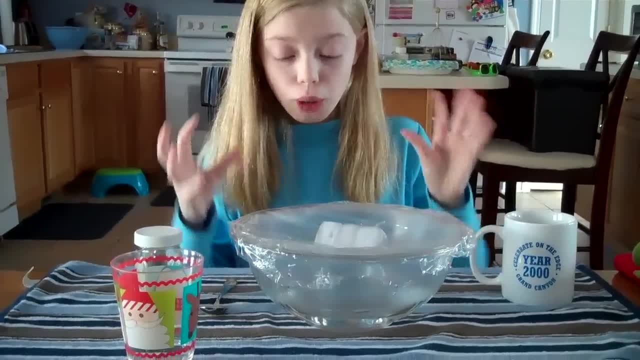 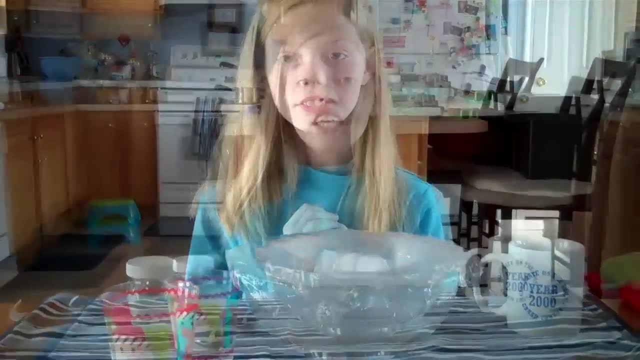 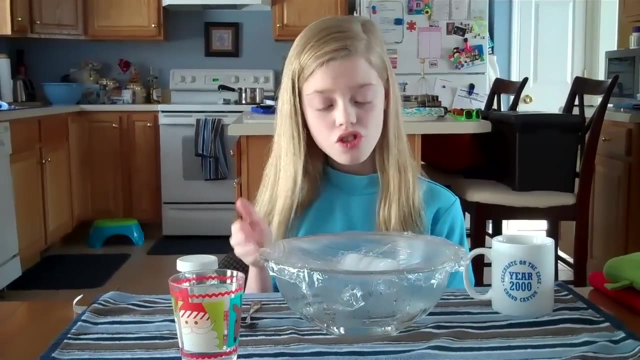 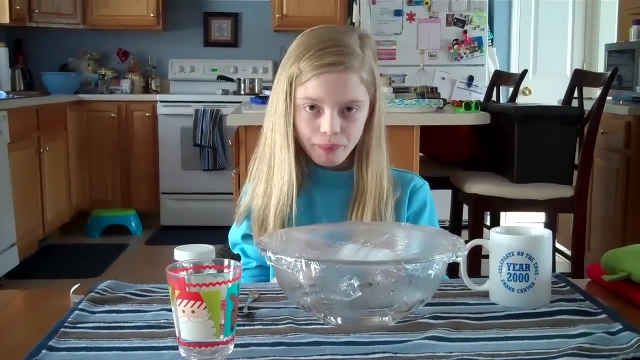 and the condensation will soon precipitate with the mixture of the cold atmosphere. It's been five minutes now since we started the experiment and there's some condensation on the clouds Now on the sides of the bowl, as you'll see in a few minutes or seconds. 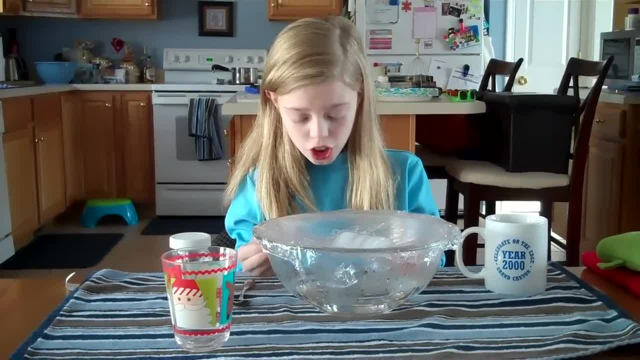 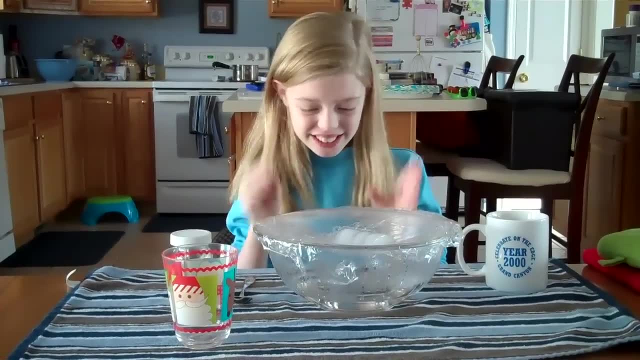 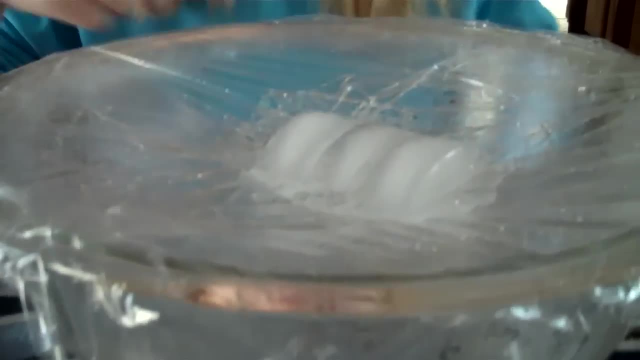 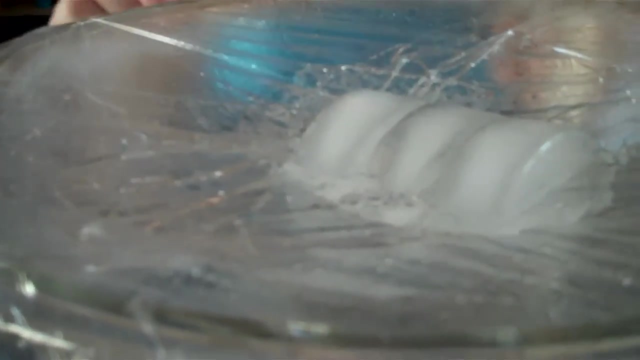 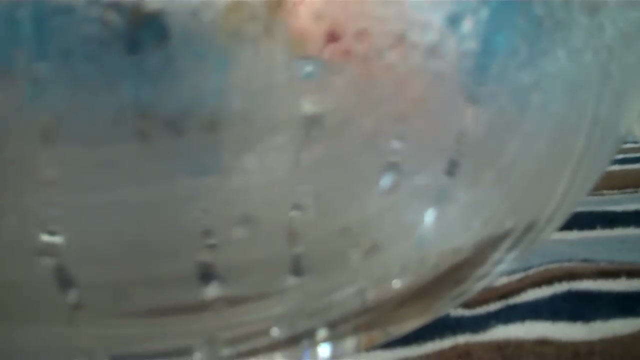 there is something that looks like condensation, that the bowl is sweating, but really it's precipitation from the clouds into the ocean. This is the condensation on the clouds hitting the cold atmosphere, creating precipitation on land. Now this looks like precipitation. 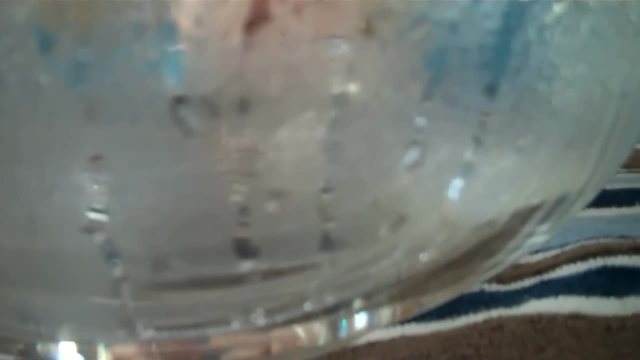 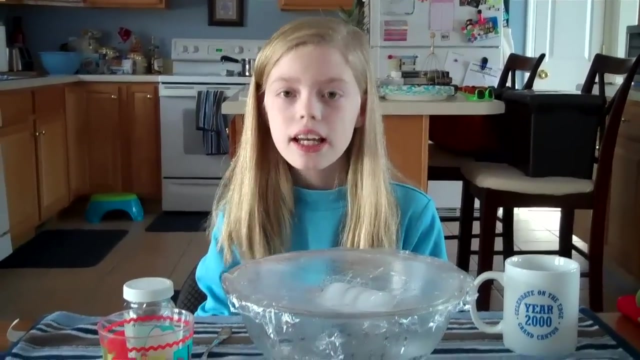 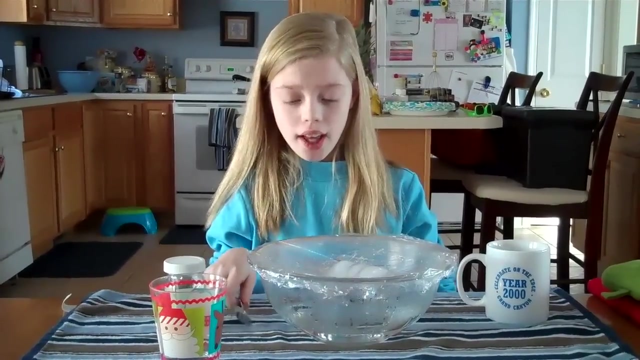 Well, it is precipitation, but it looks like condensation. Now, in five minutes we'll take off the clouds and see how much precipitation we have on land. Now it's been ten minutes and I'm going to go ahead and take off the cool atmosphere. 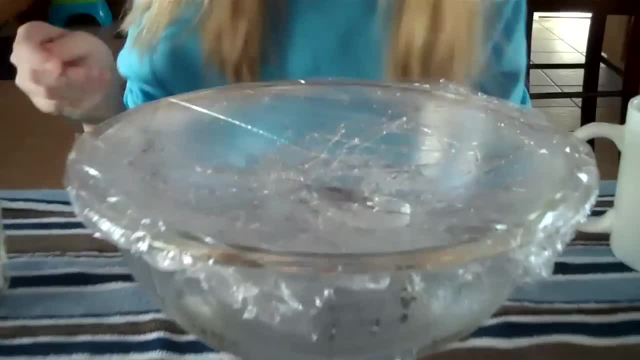 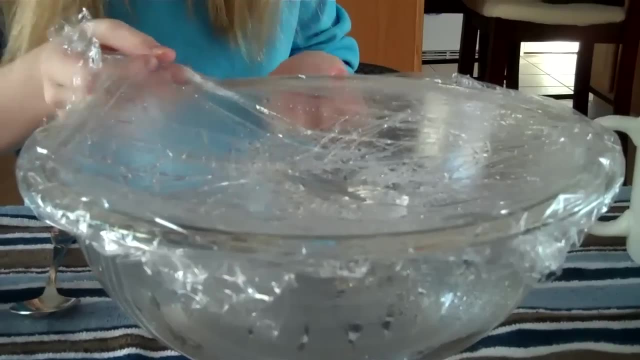 As you can see, there's a little puddle of water on the clouds, but that's okay. We're going to go ahead and take off the clouds very carefully so we don't accidentally spill the puddle of water into the land. And that was just during the whole experiment. 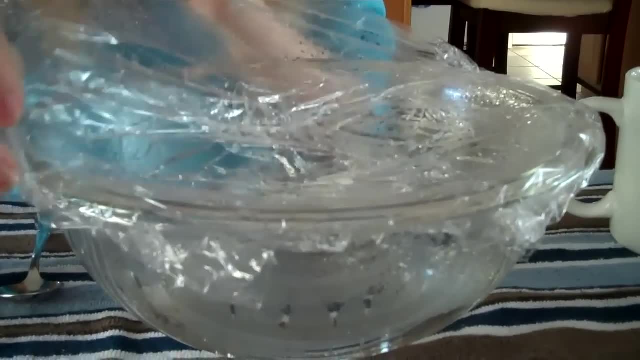 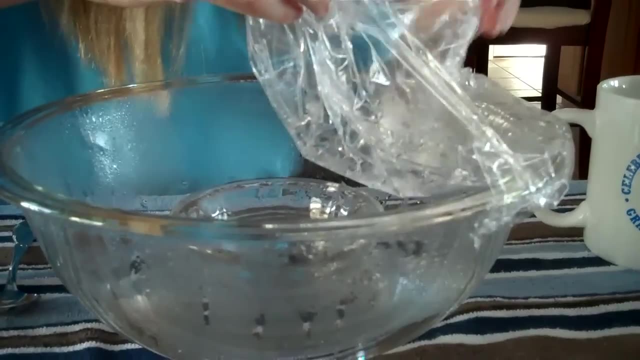 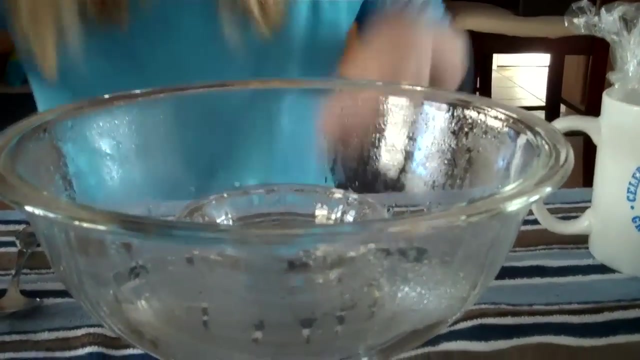 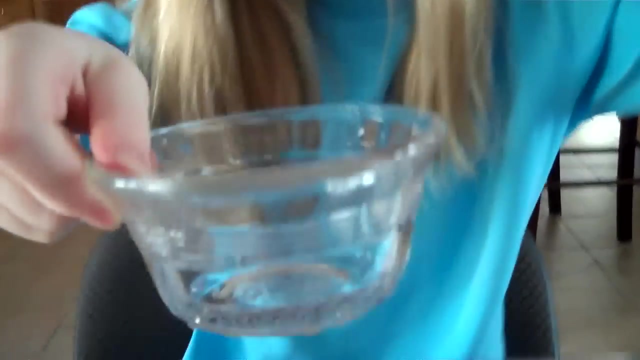 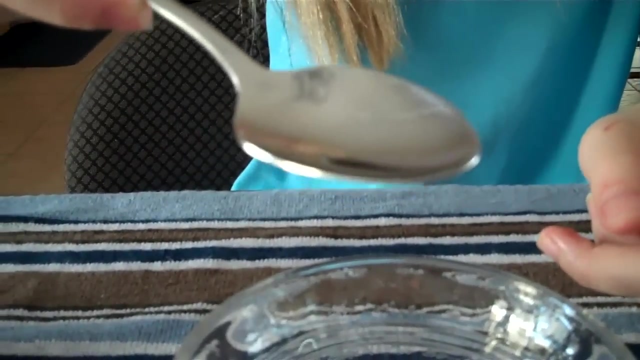 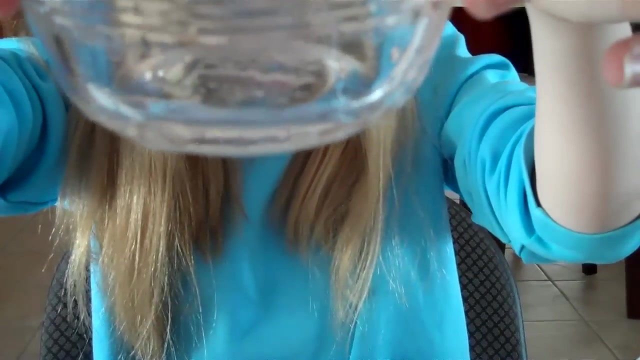 of seeing how much precipitation we have. Okay, Almost got it. Okay, Now here's the land. As you can see, there is some precipitation, Not very much, though. Here you go, I'll let you see it in the camera. 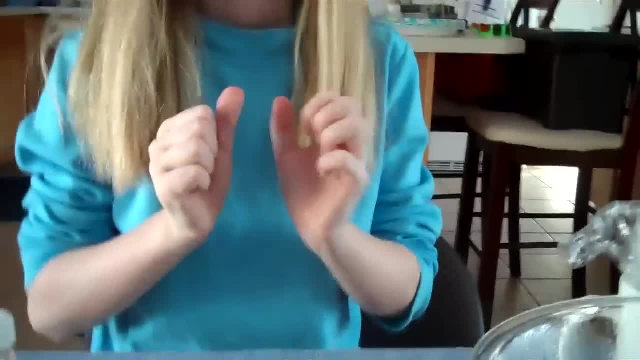 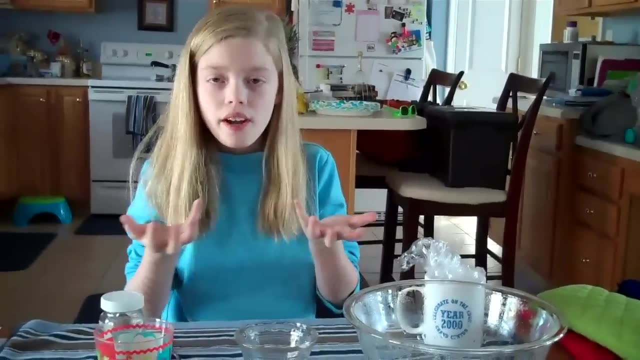 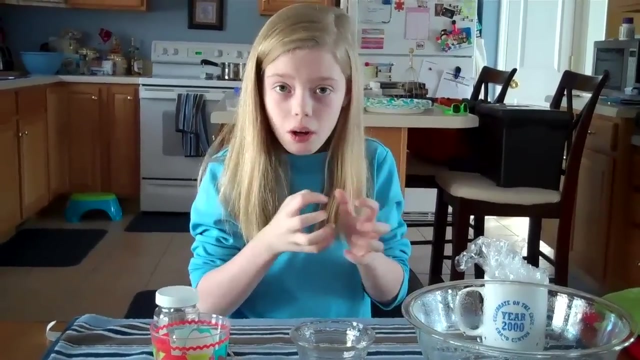 Okay, Now that is my water cycle experiment. It shows how the ocean evaporates, hits the cool atmosphere, gets water into the clouds, then it precipitates on the land. Thank you.